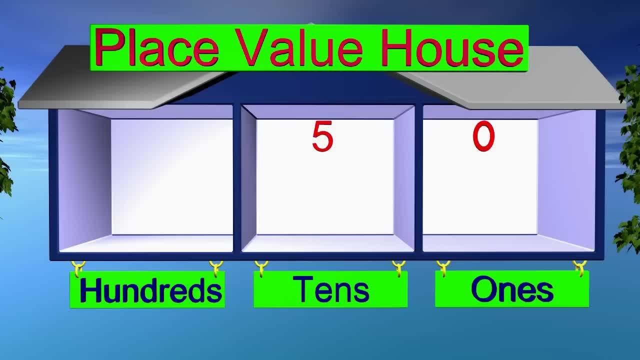 Let's look at the number fifty. using our place value blocks, We know that to get fifty we need five tens: One, two, three, four, five and zero ones. Each one of these tens blocks is made up of ten ones. If I counted every individual block. 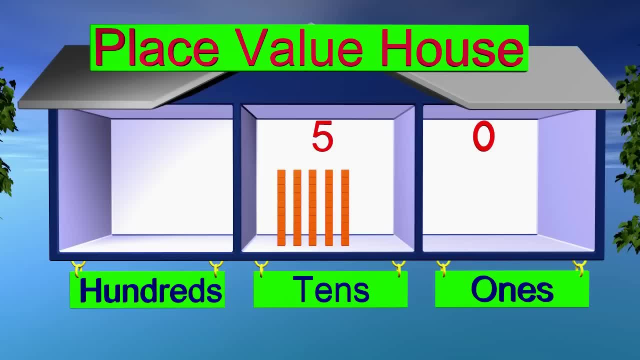 in these tens blocks, we would see there are fifty of them. Now what if we move the number five over here in the hundreds place? We cannot leave this middle room empty, so we're going to fill it with the number zero. Looking at this number: 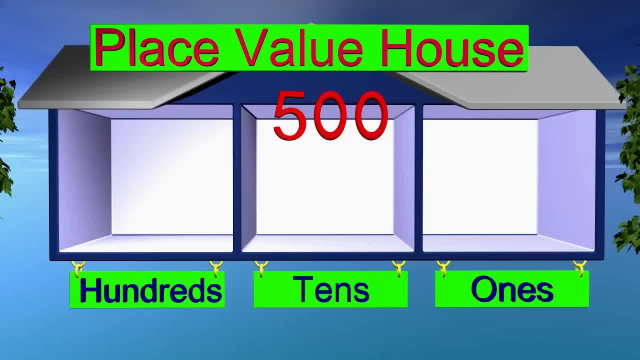 we no longer have fifty, like we did before, Is this number a lot different than fifty. With the five moving places, we now have five hundred. To show us this, let's get some hundreds blocks. To get five hundred, we need how many hundreds blocks? 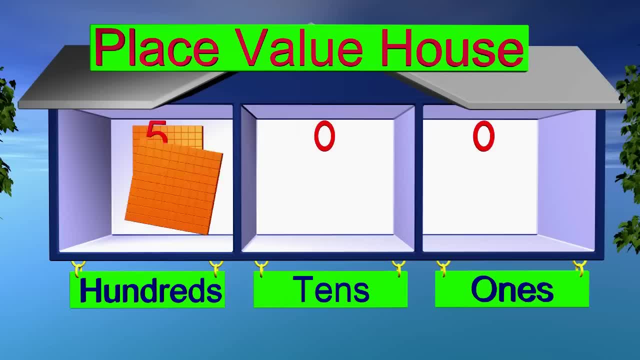 If you said five, you are correct. We need one hundred, two hundred, three hundred, four hundred five hundred. We can easily see that five hundred is a lot more than fifty. So a five in the hundreds spot is a lot bigger than a five in the tens spot. It's very important. 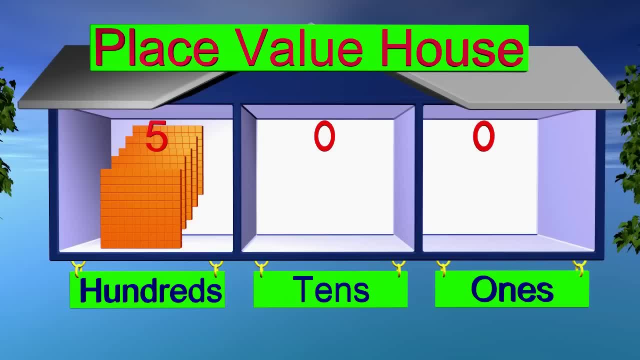 to pay attention to which spot the numbers are in, because this changes the value of a number. Let's look at another one. This is the number six and it is in the ones room. If we represent this number with blocks, we would have six ones blocks, So we have six in the ones place. 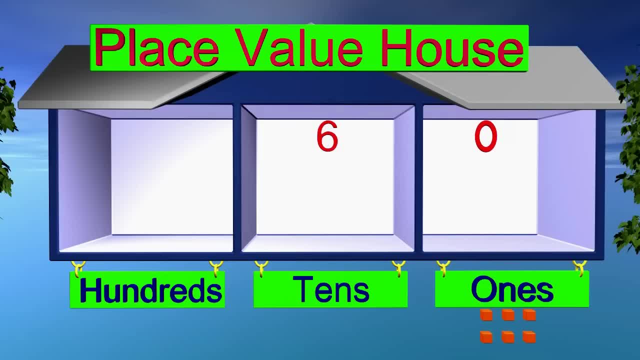 but what if we moved the six to the tens? Does that change anything? We can see the difference between the six in the ones place and the six in the tens place by using the blocks. Here we have the six ones and here we have the six tens blocks. 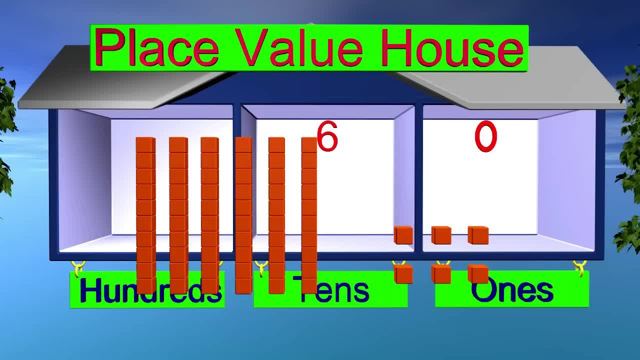 As we can see, there is a big difference between the six in the ones and the six in the tens. The six in the tens place has a value of sixty and the six in the ones place has a value of six. Remember that we need to pay attention to what place the numbers are in.